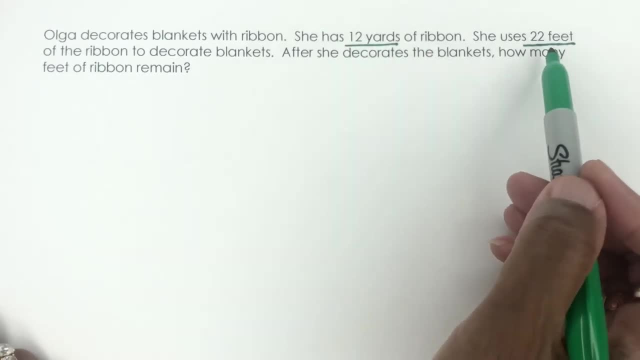 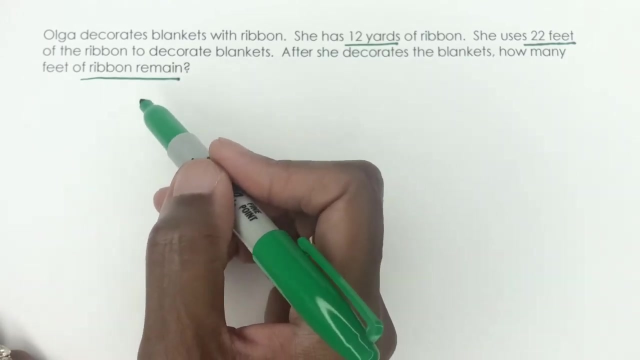 We have yards and then we have 22 feet. we need to get these measurements into one measurement. okay, then obviously the question is asking how many feet of ribbon remain. so this is an indication here. when something says how many is left over, how many is left, how many remains. so we know, we're. 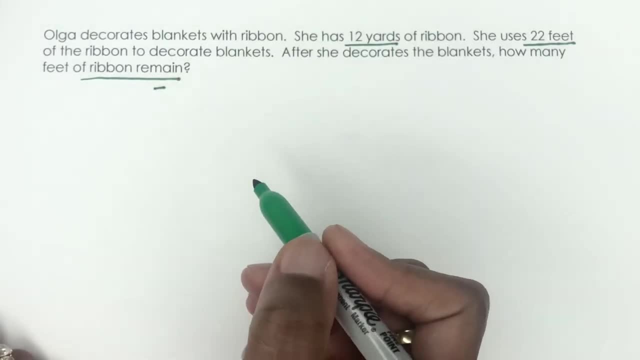 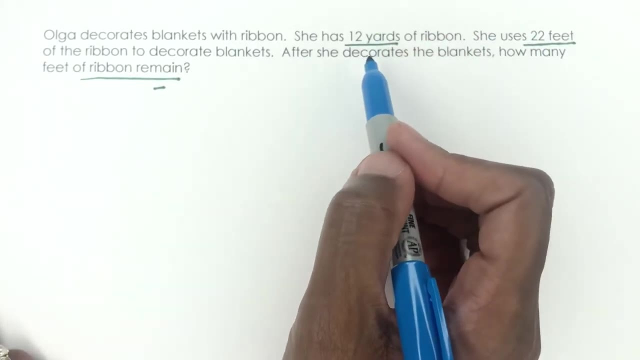 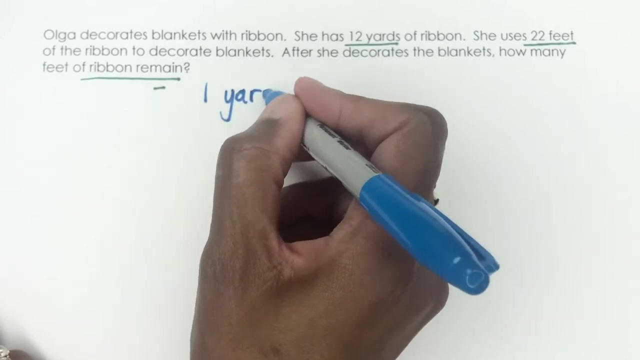 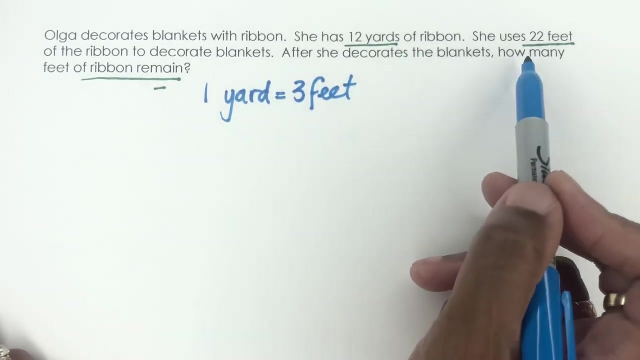 going to be using a subtraction at some point in this whole calculation. so the first thing we have to do, guys, is we have to change our yards to feet. you remember that conversion. let's do it here. so one yard is three feet. so if one yard is three feet, we want to get the whole thing in feet, right? 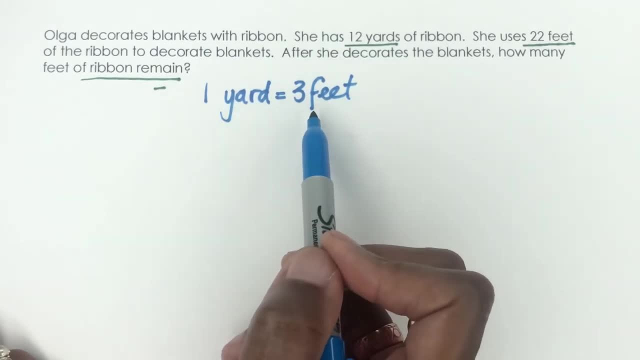 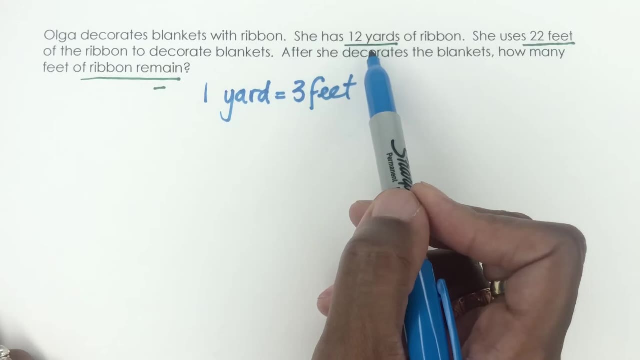 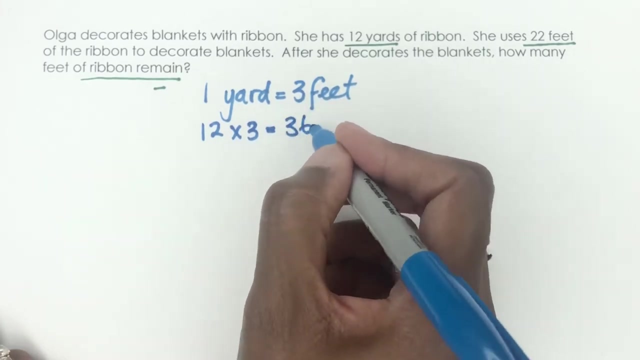 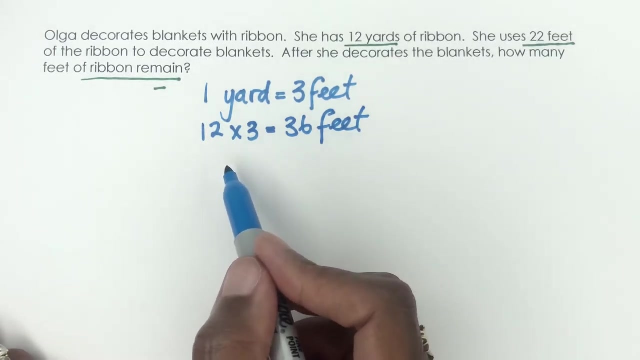 so if one yard is three feet, how many feet right do we need for 12 yards? so obviously we're going to multiply that by three right? so 12 times three would give us 36 feet. now how do we know to multiply? well, you can also do a, what they call that proportion. so you could say: one yard is three. 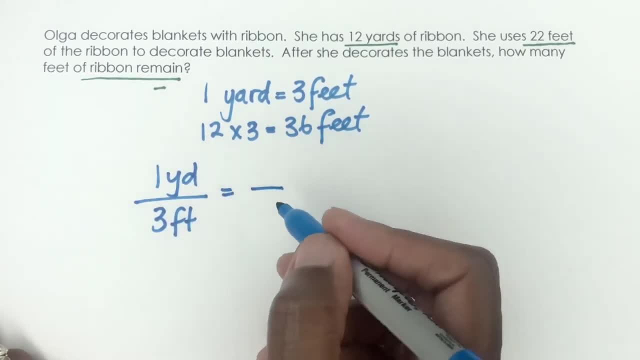 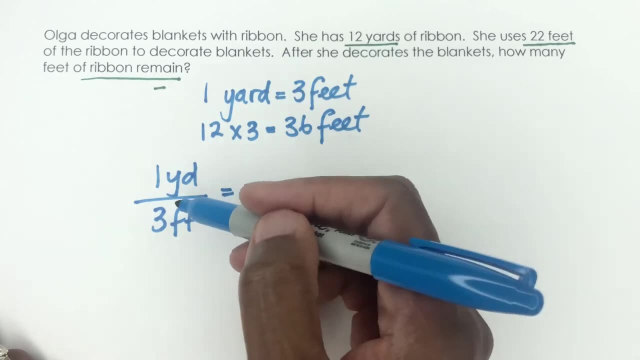 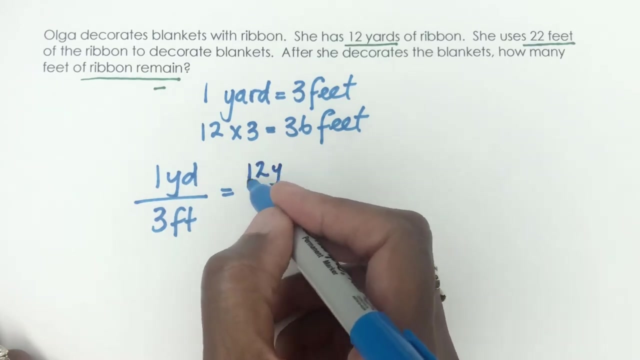 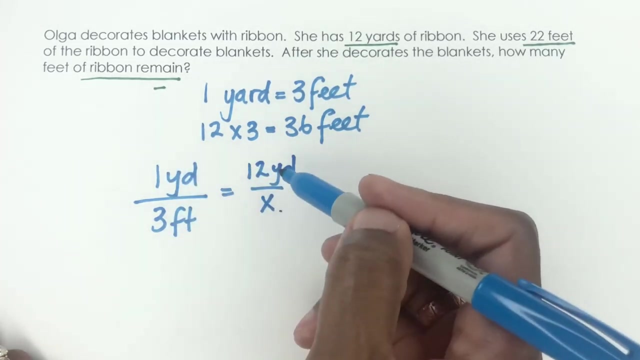 feet, and then proportion means you have to keep the same measurement. so yards is upstairs and feet are going to be three feet. and then proportion means you have to keep the same measurement, so yards is upstairs and feet are downstairs. so if one yard is three feet, then what is 12 yards? so yards is up here, so you're going to put the 12 up here with the yards, right? so then we're trying to find it out down here. then, right? so then you would do a simple cross multiplication, right? so three times 12- that's why we're multiplying- three times 12 is 36. that's how we got the 36 feet right, okay? so then once we've done that, so the next thing to do then 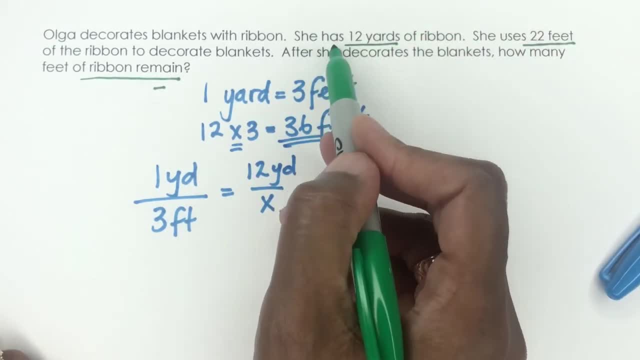 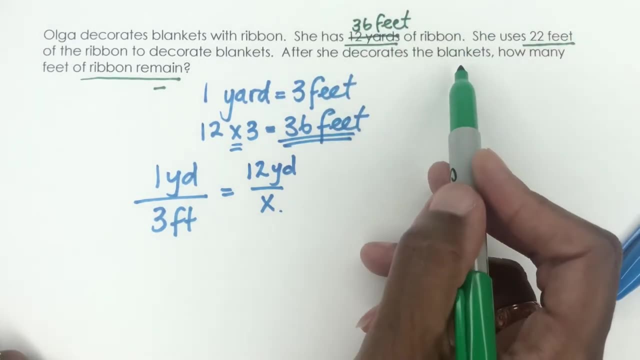 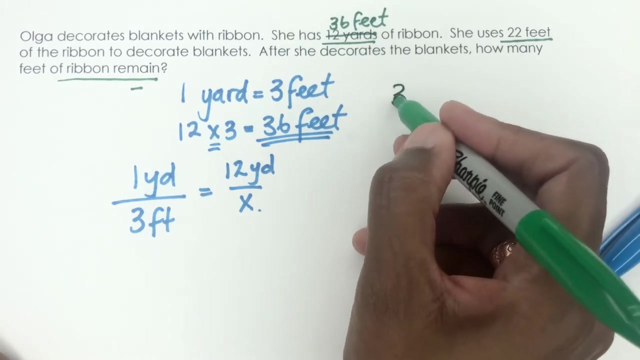 is to change this. so she has, Olga has- 36 feet of ribbon and she uses 22 feet. now it's going to make it easier to do now, right? so then we're going to say 36 feet minus 22 feet, and we know we're minusing because it.